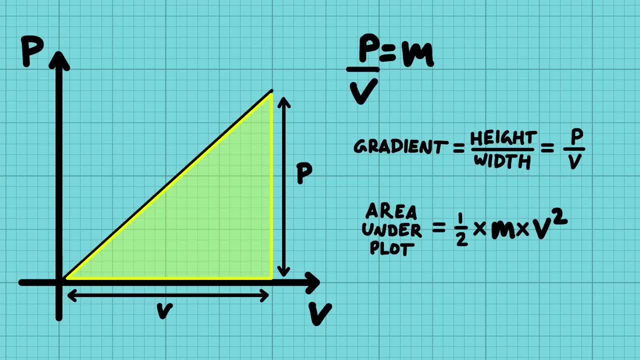 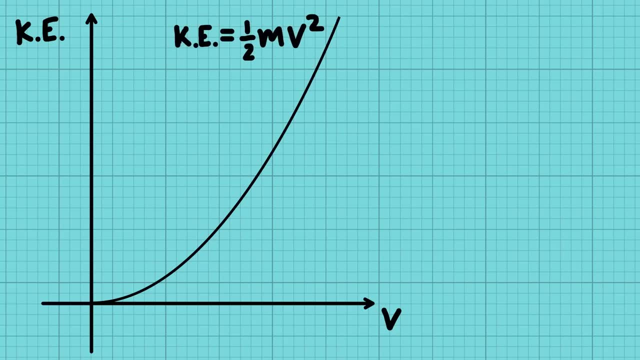 It's just the height divided by the width of the triangle, which, in my example, is the mass m. Things get more difficult when you've got an equation that's got a curved line, like the plot of kinetic energy that we've derived. It's a curved line because it's got a v squared in it. 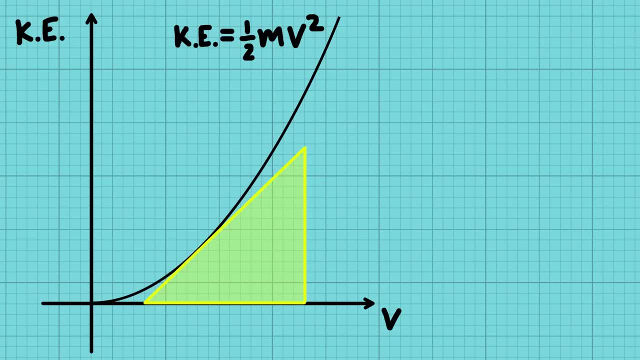 Now you can't just use a simple triangle to find the area and gradient. You need to use integration and differentiation. Now I don't have time to teach you all of calculus in this video, but I'll give you a brief description of the way it works. 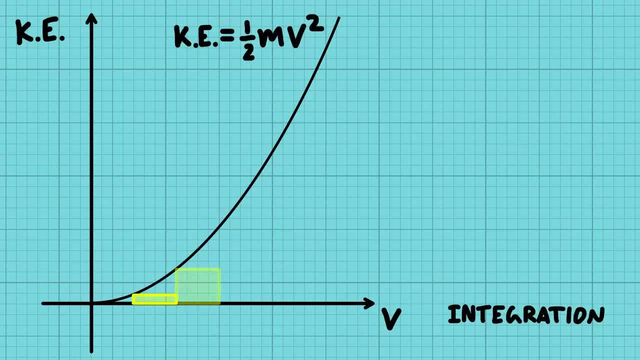 The idea behind integration is that you start by approximating the area under a plot with a series of rectangles, So we can write that each area is a half mv squared, which gives the height times a small width, which we'll call delta v. 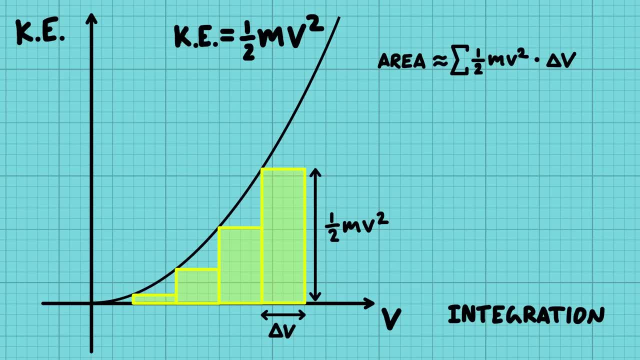 And the total area is the sum of all of these rectangles. The trick to integration is that as you reduce the width of these rectangles to be smaller and smaller, this approximated area gets more and more precise and becomes perfect when the width of the rectangles gets infinitely small. 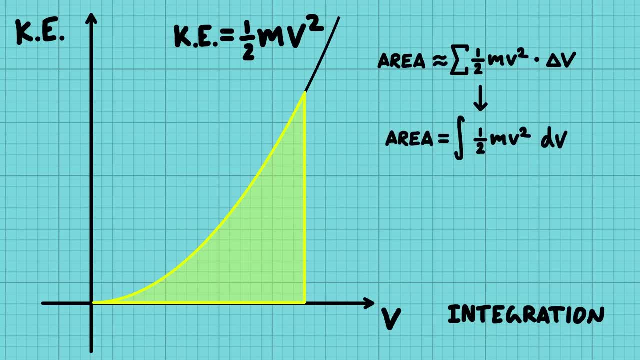 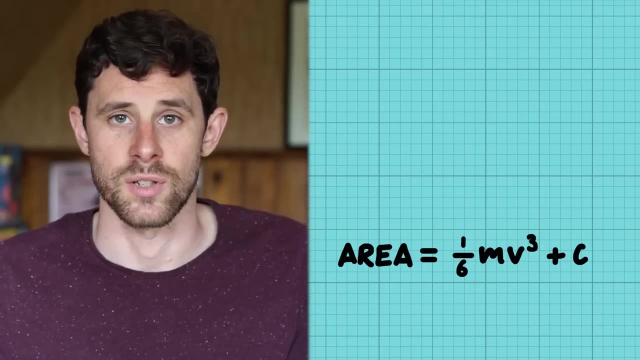 Then we rewrite this sum as an integral, which looks like this: If we do this integration, we come up with this equation, and this is already kind of interesting because as physicists we don't have a name that describes the quantity, So we're already sort of in the wilderness of physics. 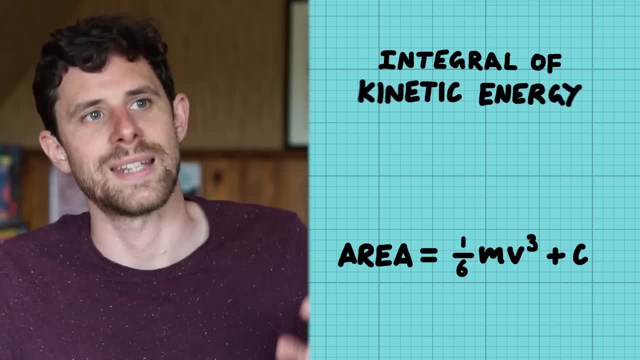 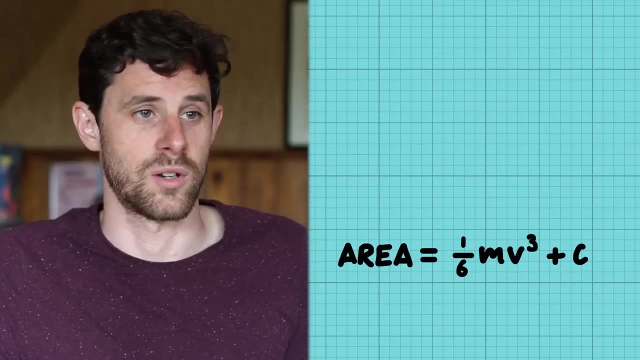 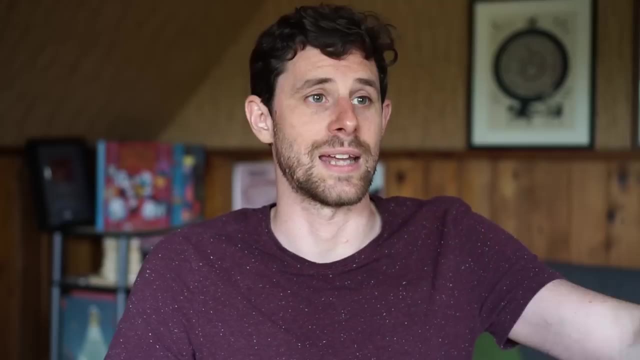 A physicist's description of this would be the integral of kinetic energy with respect to velocity, But seeing as we've discovered it, we can call it whatever we want. So we could call it like superkinetic energy or something, And that's basically what happens in physics when physicists get to a new concept. 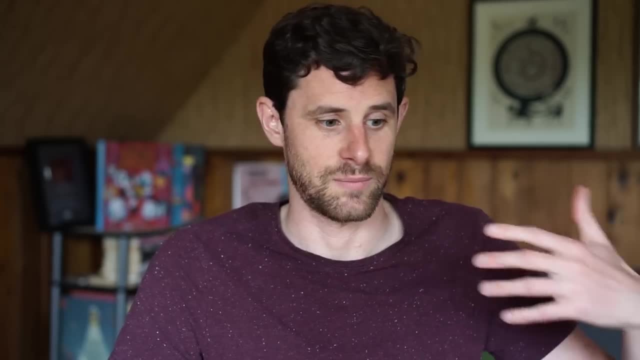 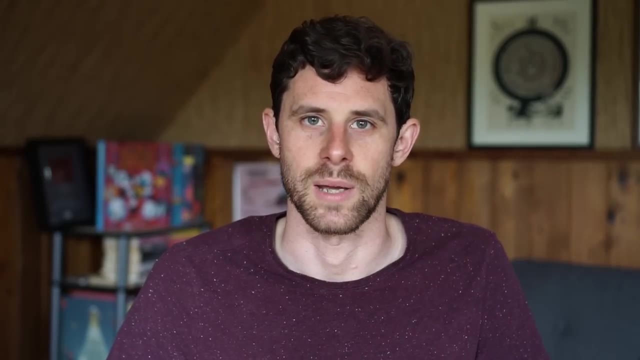 They've got the job of describing it, Which is why physics is sort of got so many weird words in it, But there's nothing special. it's just people naming stuff. there's nothing mysterious about it. Differentiation is sort of the opposite to integration. 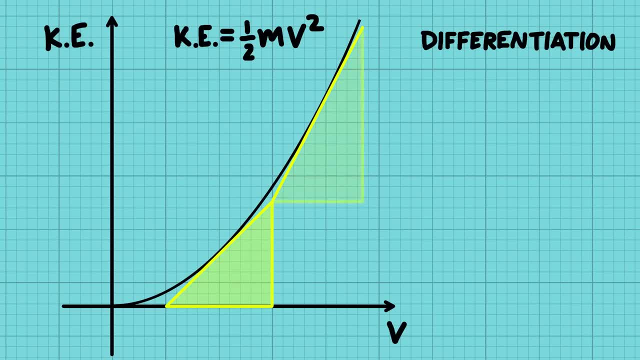 Here you approximate the gradient with tiny little triangles at each point. So we would write that the gradient is a delta half mv squared divided by delta v. Again, the approximation becomes perfect when these triangles are infinitely small. And then you write out a differential equation which looks like this: 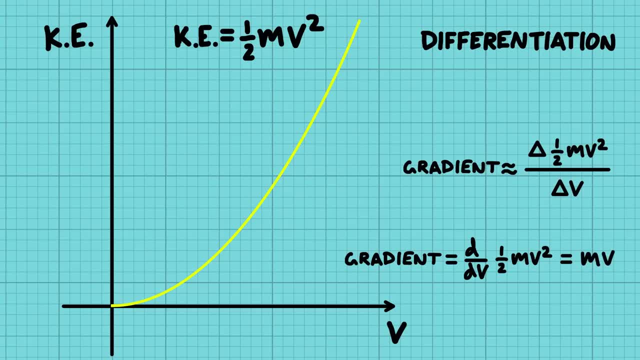 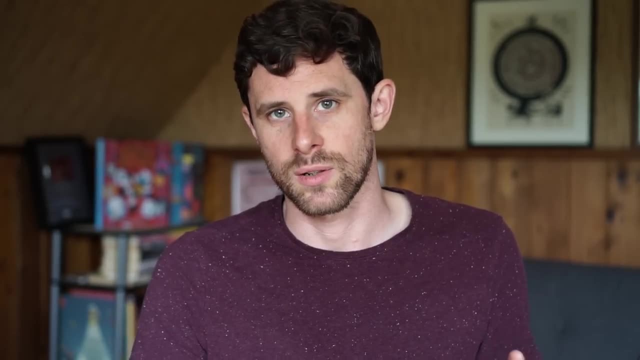 The solution to this equation is mv, which is basically back to where we were at the beginning of the video. So differentiation is a kind of inverse or opposite process to integration. That just gives you a flavour of calculus, But if you want to find out more, there's a really good playlist on calculus on the channel 3Blue1Brown which you can get up here. 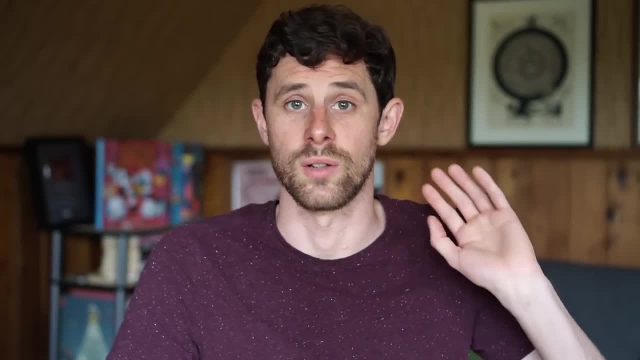 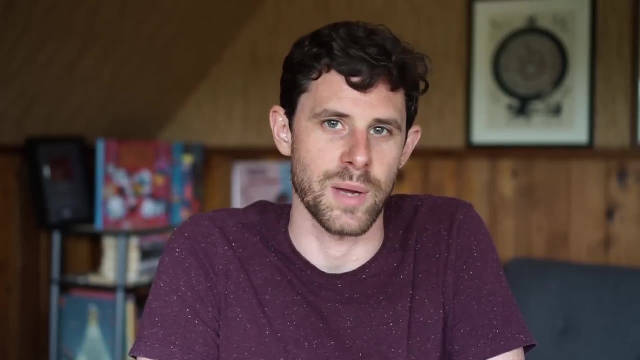 I really recommend it. it goes into way more detail And in fact the whole channel I love. it's so good. So calculus is normally taught as kind of an abstract set of mathematical rules, But to a physicist it's kind of the bread and butter of what we do day to day. 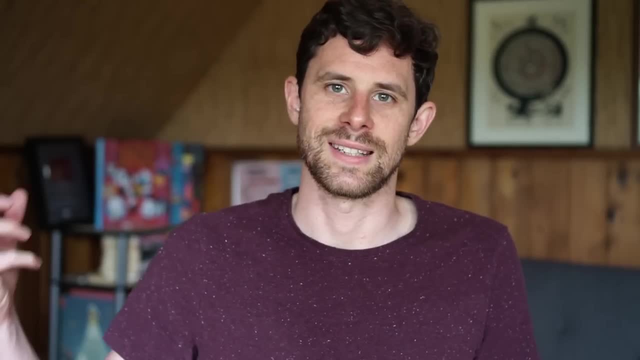 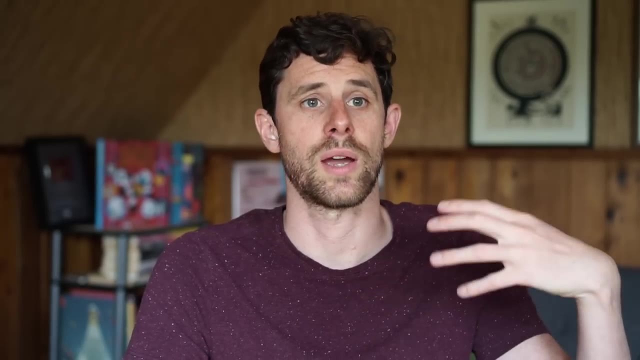 You know, like a plumber has got a wrench, a physicist has got calculus, And when you learn physics in school you're given a bunch of equations and you have to memorise them and you have to apply them in different ways, But you're never really told where those equations come from. 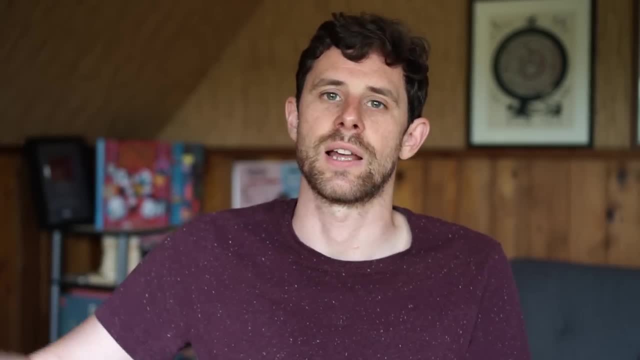 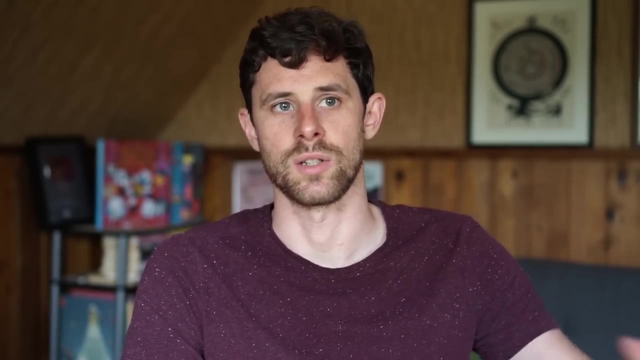 Which is understandable. you don't have time when you're in school and it's kind of like a next level understanding thing. But when I was at university and I learnt calculus and then I learnt the derivation of all of those physics equations, it was a really satisfying thing to learn because it was the first time where I really understood kind of why those equations existed. 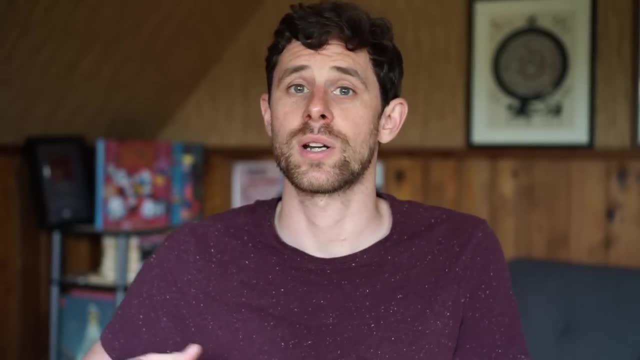 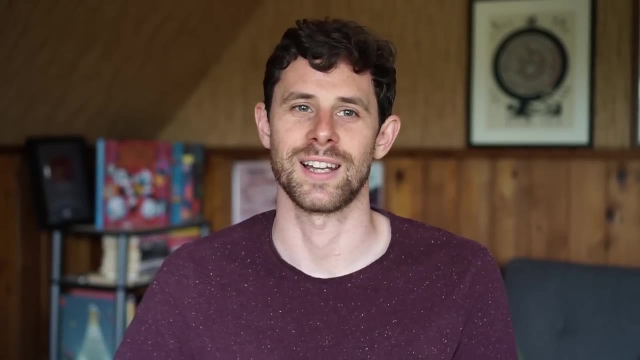 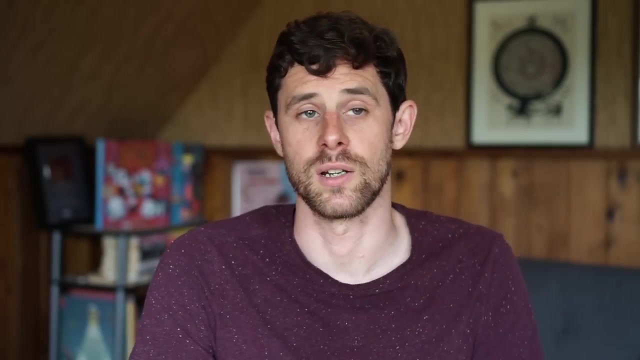 where they came from and also how they related to each other. And then, when I started being able to apply calculus to come up with my own equations, that was incredibly cool, Because it's like you're a freaking physics wizard or something, And so if you ever get the opportunity to learn calculus, I really recommend it. 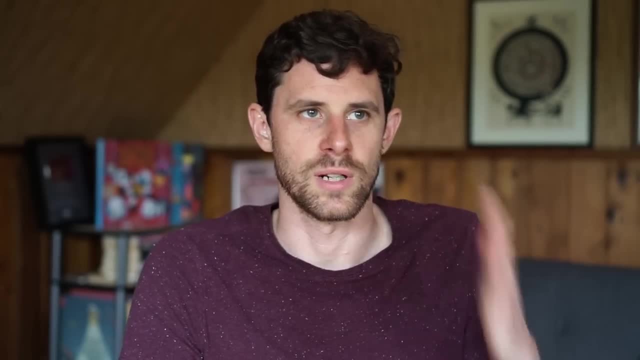 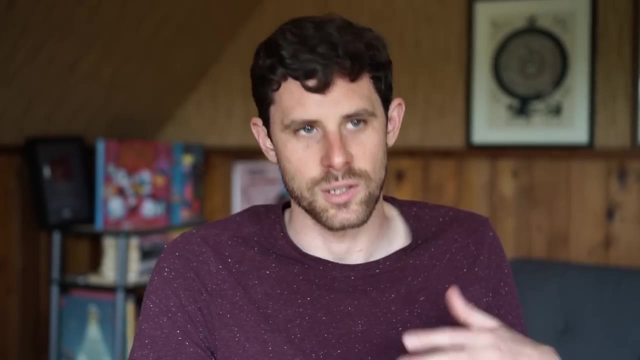 Even if just for your own interest, it's definitely applicable. And if you're learning calculus and you don't really know what the point is, learning something that gives you the ability to derive new physics is a very good reason. I should mention that algebra and calculus aren't the end to the mathematical tools. 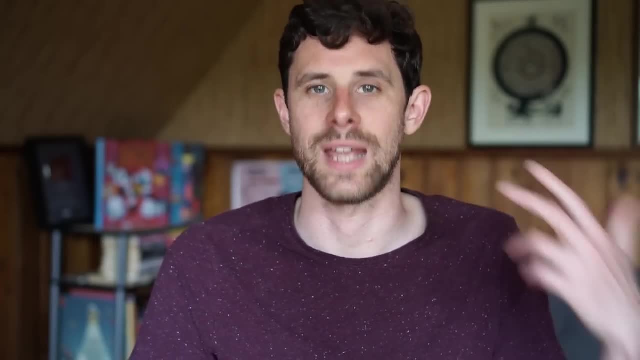 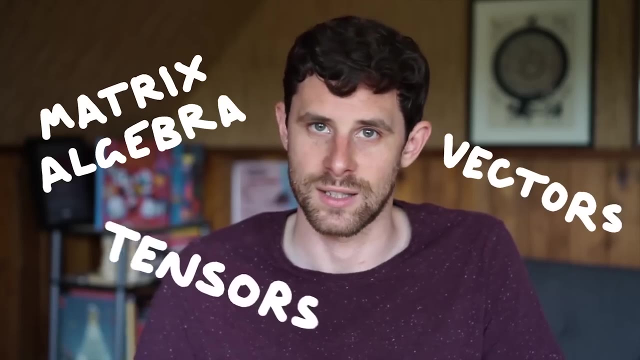 That physicists use to derive new physics, but they definitely form a foundation which then you can build upon later or add on different things like matrix, algebra, vectors and tensors. Depending on what path of physics you go into, you'll need different kinds of mathematics.